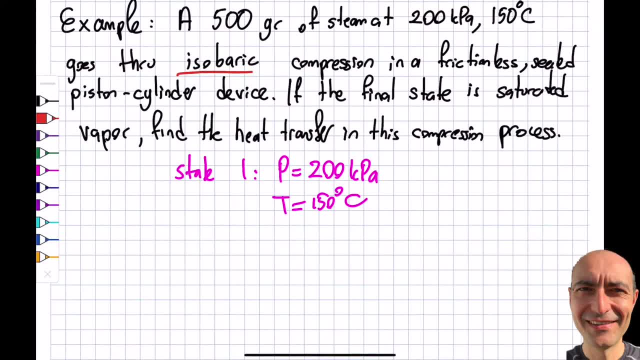 So state two goes through isobaric compression. Okay, isobaric means this P is constant. So if so, then if I look at the state two, then my P will also be 200 kilopascal. as the isobaric name indicates, It's a frictionless sealed piston cylinder device If the final state is saturated vapor. So what it's saying is state two is P is equal to 200 kilopascal, So it means it is the saturated pressure. 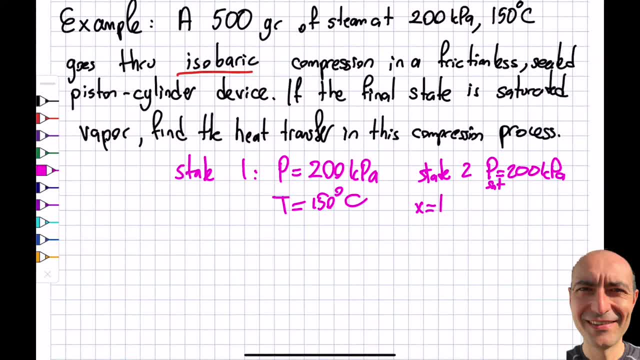 And if I, x is equal to one, which means that this is saturated vapor, right, I have 0% saturated liquid, I have 100% saturated vapor. So if I represent this like that, so this is going to be T, it's going to be, let's say, V. And if I have something like that, right, and constant pressure lines are like this, do you remember? So this is the point that I'm at. That's what it means. I'm at the saturated vapor. Okay, All right, And obviously this is 200 kilopascals. 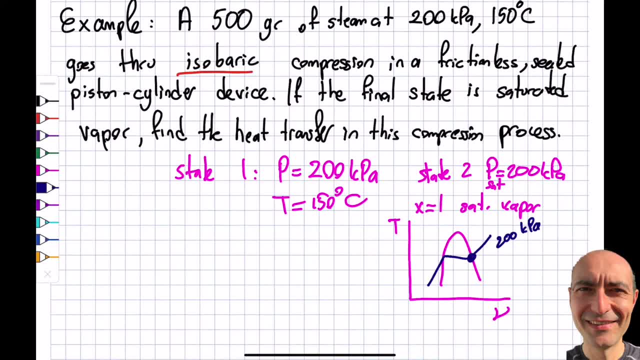 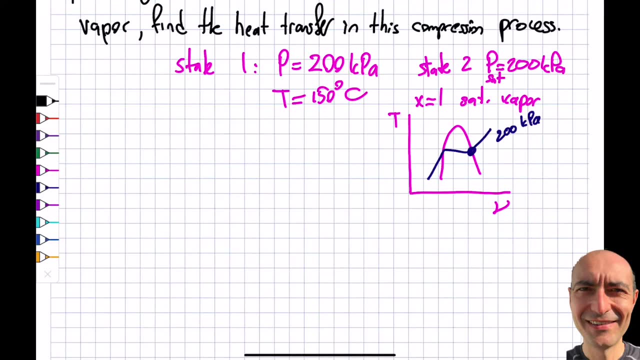 Okay, so I made enough point about that. Find the heat transfer. So actually I did visit this question before I was looking at the boundary work, So now I'll do the whole whole thing to illustrate. Okay, So whenever a heat transfer is asked, so they basically means that so far we only covered the first law. right? It's an energy balance. So let's go ahead and write that Q net minus W net will be equal to delta E of the system that we have. 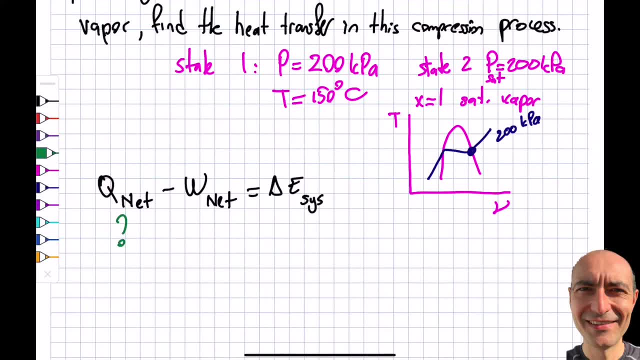 So the Q net is indeed the question mark that I have here. Okay, So what about the work net? So that is actually coming from the previous module. we will have W out minus W in plus boundary work. This is my W net, Okay, And delta E of the system. So I want to make a point over here. I have a cylinder, piston, cylinder device, right? 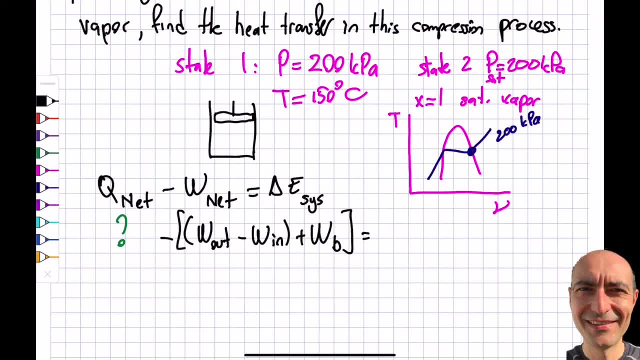 And this is sealed. And what is happening is, if I have myself a control volume- in this case is called control mass because it is sealed, right? So this is not going anywhere. It is stationary. It is changing shape though, right? If I'm compressing this from state one to state two, right, What will happen is this will go down, So the control mass will be squeezed, But at the end of the day, it's not going anywhere. Okay, those are two separate concepts, So let's not confuse those two, Okay, 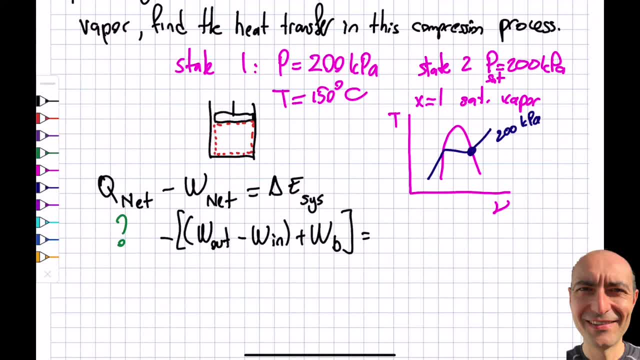 Okay, If this was a moving control mass or control volume, you cannot assume a stationary as this. just the shape is changing. I should be able to go ahead and use a stationary, So let's write it in here. It's stationary, So that means it's going to be U2 minus U1. That will be what it is, If I want to write this in terms of the specific internal energy, because these are given in the charts, or rather the tables. So let's take a look at the 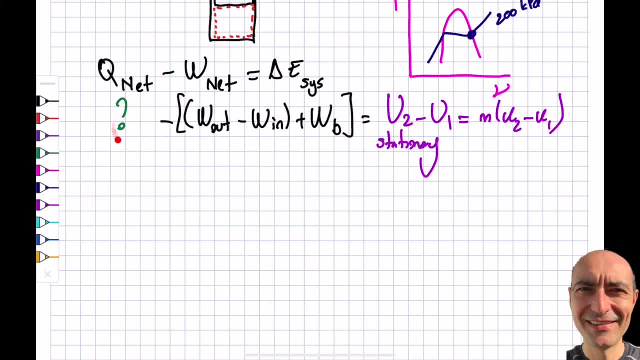 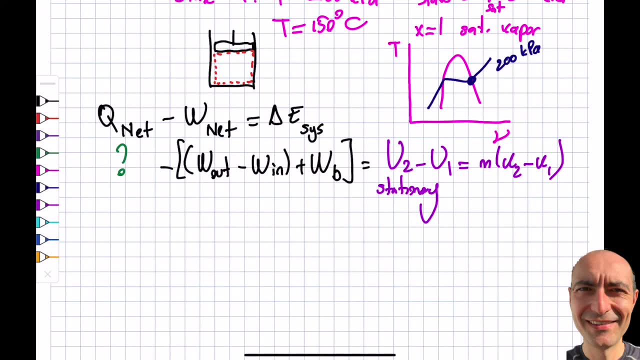 terms before we go proceed. So this is what I'm after. There's a minus sign W out. Okay, the question is, when I'm looking over here, is there I have something like a turbine connected to, so I take some kind of workout And not really. What about some kind of a propeller that is coming into it as an example And it just, you know, in putting some type of work into the system, like it's rotating as an example? No, I don't have that either. Okay, What about WB? I did visit this before And I will. 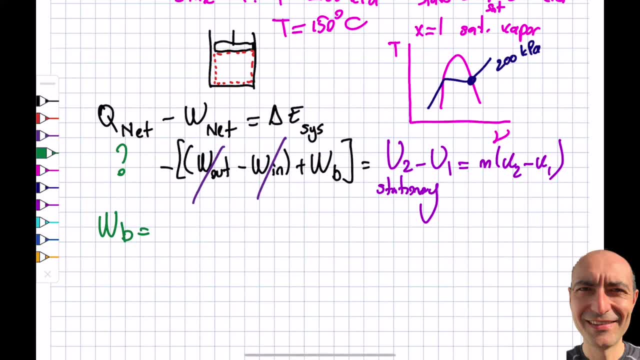 put a link right over here, Okay, But this WB was integral of P TV. Remember that for constant isobaric process, we said that it's going to be P times B- two minus V one, And also I said that this is going to be P times n times, specific volume: two minus specific volume number one. Okay, And the good thing is, let's take a look at this here. So I'm going to just take it and plug it into here, And the only thing I don't know about here is this too, But as long as I have my states, 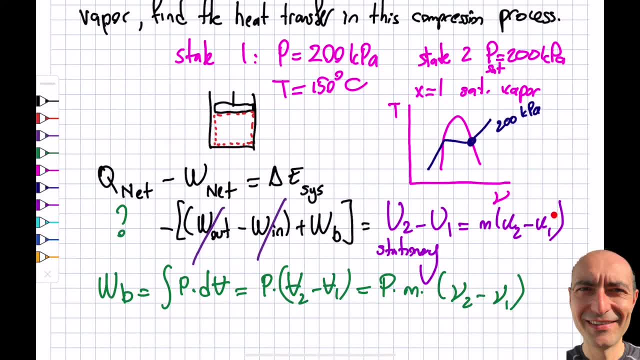 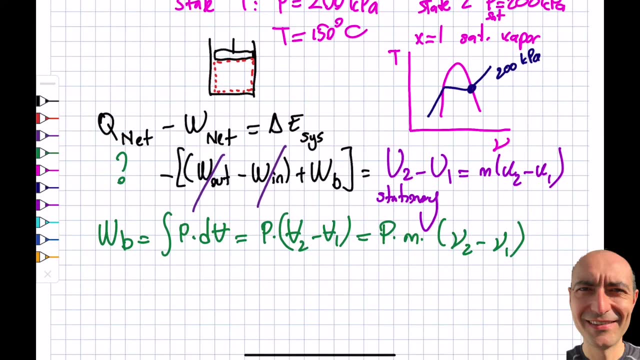 and you can see over here my states are defined, So I should be good to go about this same logic wherever I'm looking at this, you know, simply go ahead and note down my specific internal energy as well. Okay, again, as I said, I will link a video here And I'm not going to go in that. But you can watch that particular video. But the state one turned out to be a superheated vapor, if you remember, And for that I go to a six of 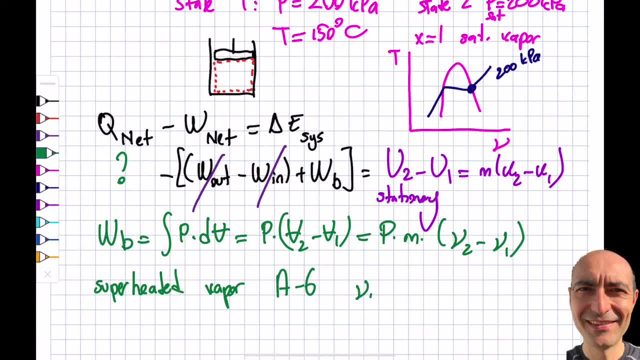 Chengel 9th edition. right, And I note down my specific volume. one is 0.95986 meter cube per kilogram And I get myself you want while I'm at it. why don't I note that down right: 2577.1. 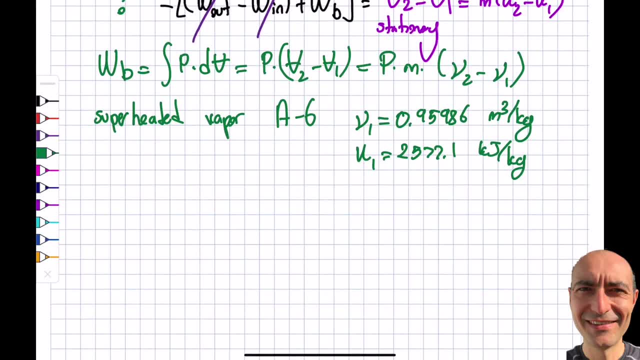 kilojoule per kilogram. Okay, let's take a note over here. You see the kilojoules, not joules. joules is too small, So this is actually 2.5 mega joules, right? So it's pretty big, right? So? 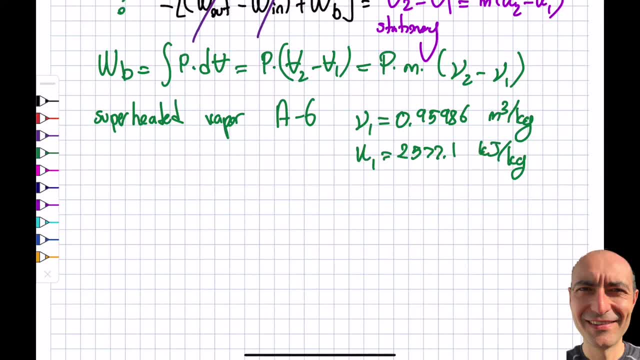 I have to be consistent and be careful about these things. Okay, What about the second? So let's call the state one. Let's look at the state two. Now, state two is actually a mixture, right? So I have actually x is equal to one. So I simply like to go and look at this: VG at 200. 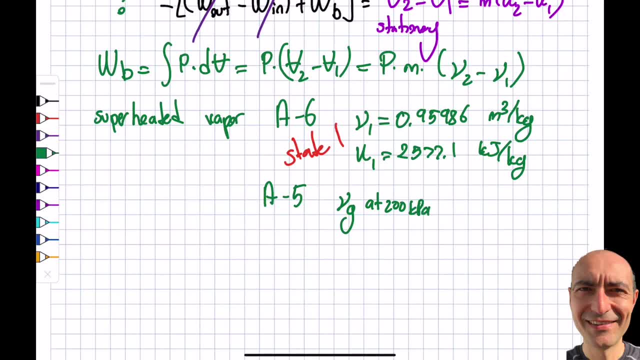 kilopascals. right, And if I do it I will see myself, as this is going to be the second one, that will be 0.88578 meter cube per kilogram. So that is so far, so good, And I also have the. 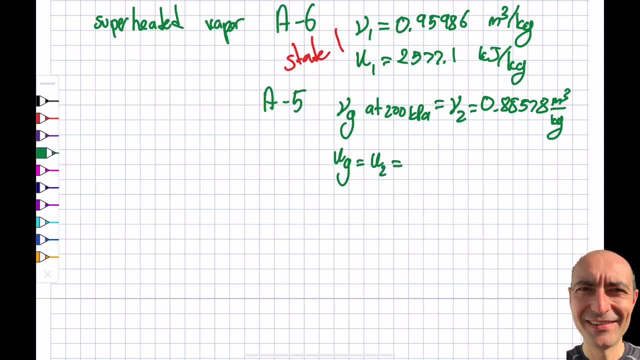 same thing, ug will be equal to u2. from the same logic, I'll get this 2529.1 kilojoule per kilogram, So I'm actually in a pretty good shape, if I'm not mistaken, because I don't know this. 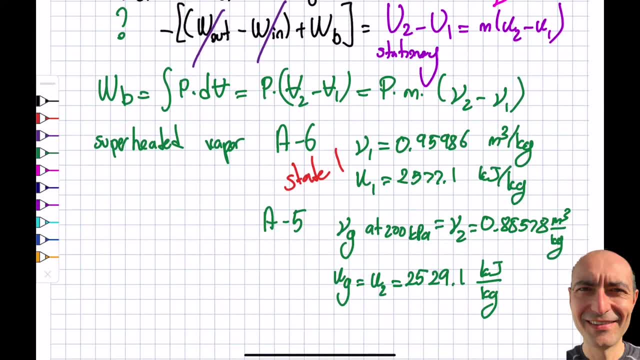 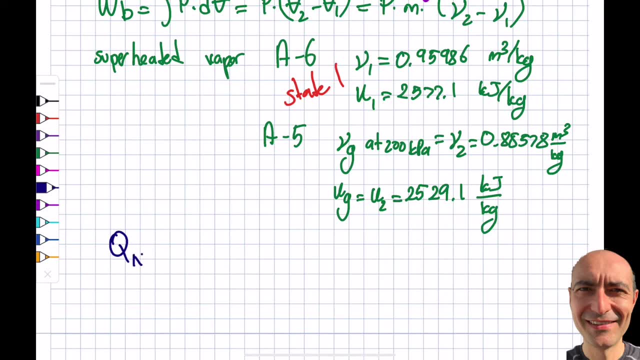 right, That's what I'm asking, But this seems to be, you know, pretty well formulated. So why don't I go ahead and write this one more time, just to save, or rather just to show you, because I'm going to make a point. I see this sometimes, You see, do not forget. 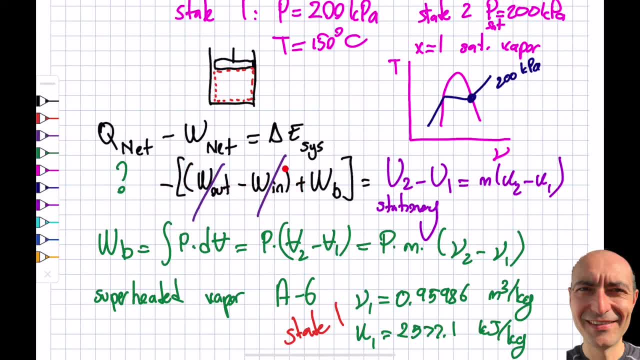 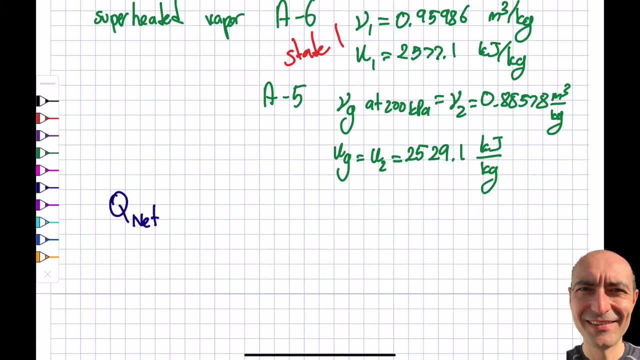 the negative. okay. Sometimes students put a negative only in front of these parentheses and add a plus. that's not quite correct, right? This is a bracket, big bracket, be careful. So q net in this particular question, q net minus WB is equal to m times u2 minus. 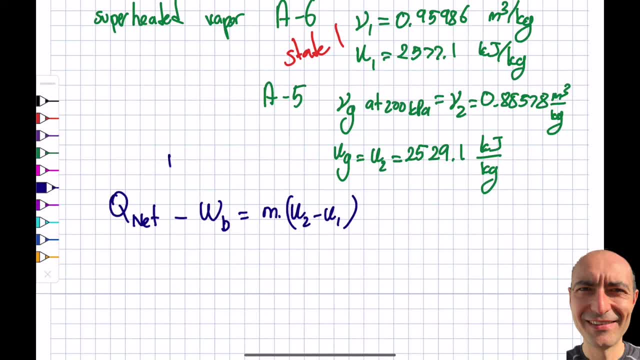 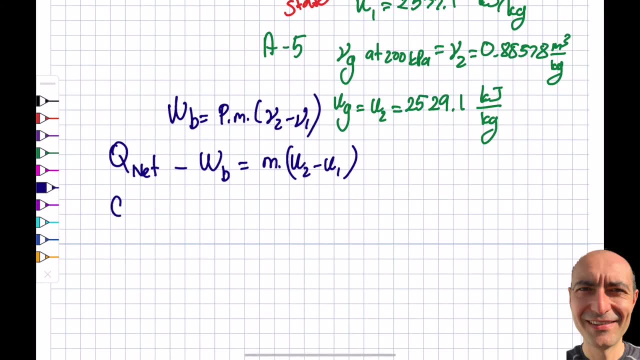 u1, right, Okay, okay, And this WB turns out to be p, m, v2 minus v1, right, So I'm going to use that information. q net minus p is 200.. Okay, you have a choice here. You can use everything. 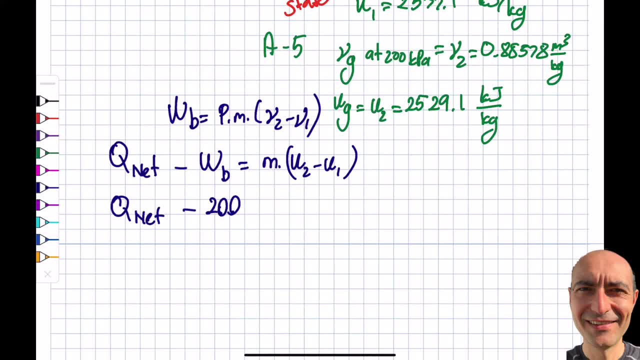 with respect to joule, which is the SI, and then you need to turn when you go to here. you need to convert this to joules, not you cannot write kilojoules, Or I'll take that second pad for this particular question because I showed the other one quite some time. 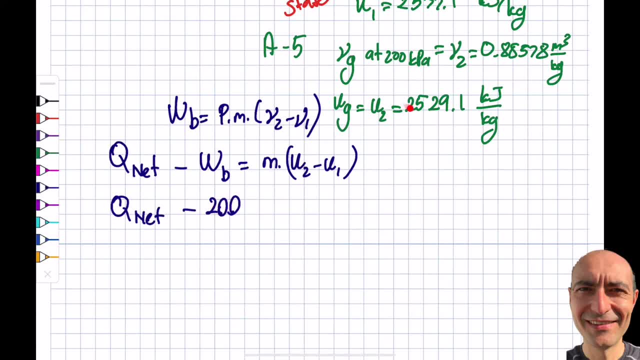 So I can actually use this pressure to be kilopascal. as this is kilojoules, where is it Kilojoules? I will be able to be consistent in my units as well. That is up to you do. 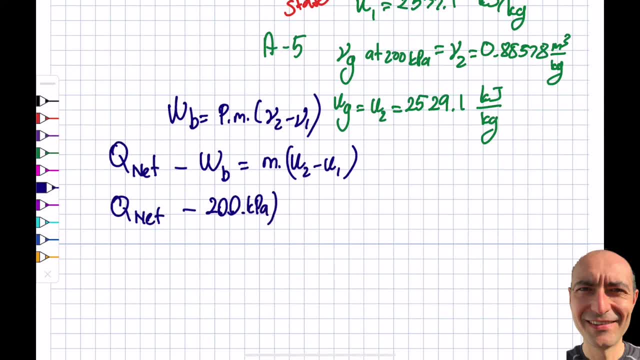 what you got to do. okay, So this is in terms of kilopascals. I have the mass is 0.5 kilogram and I have this v2 minus v1, 0.88578 minus 0.95986.. And, if you remember, this was meter. 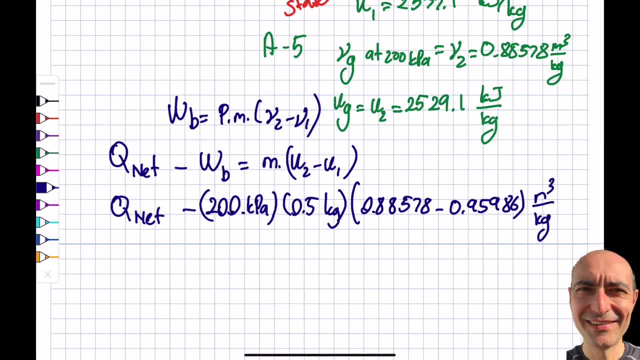 cube per kilogram. okay, Again, I did this in the previous segment too, but you can see this is kilonewton per meter square, so the meter cube and meter square will cancel. I'll have a meter in here. kilograms cancel, so I get a newton meters. this is joules, So again, I have a kilo over. 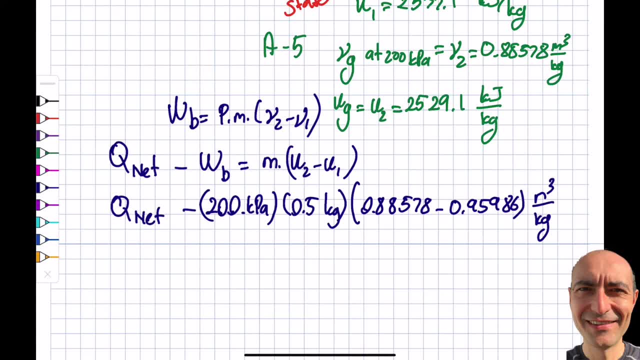 here. so I'm going to get kilojoules, so I'm doing something right over here, okay, So let's look at the right-hand side of the equation, and that will be m, which is 0.5 kilogram. so I have to write this in terms of the kilojoules which I will. 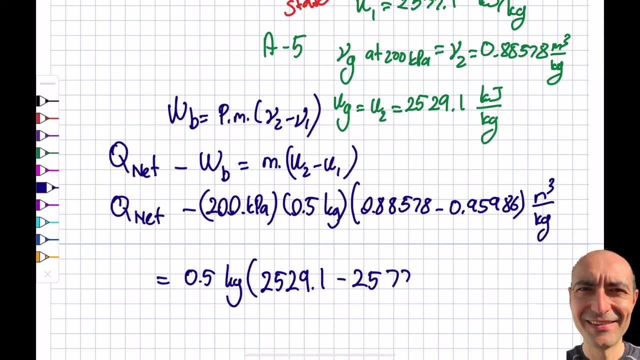 0.95971 minus 2, 5,. I think it was 7, 7.1,. I'll check and come back. Yep, that's correct, And this is also kilojoules per kilogram. so good, So I have this in terms of the kilojoule.